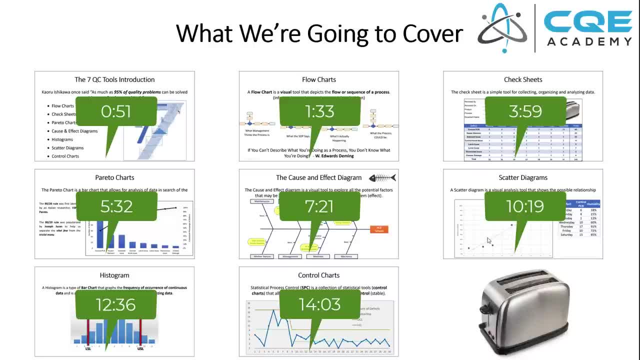 and then the control charts, And then along the way as we go through this, we're actually going to work a problem using all seven tools and we're going to reduce the number of defects associated with our toaster. All right, let's go ahead and get started. So the seven QC tools: 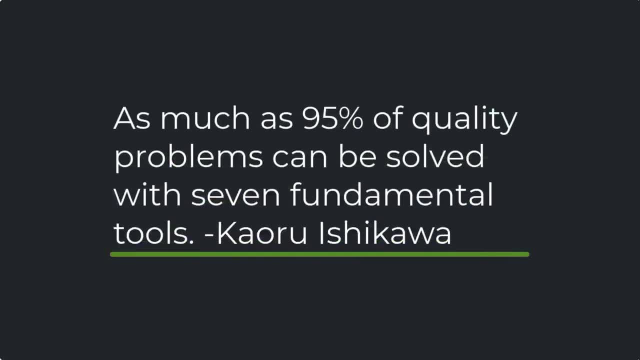 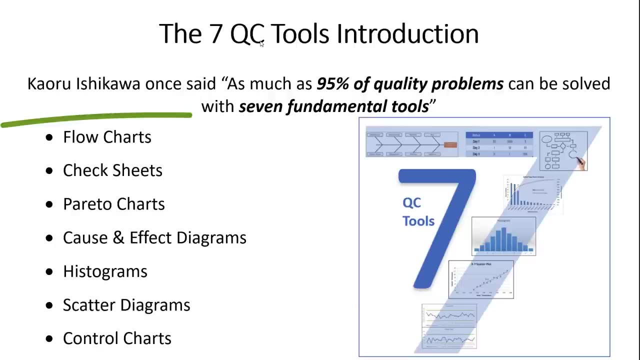 I love this quote from Keoru Ishikawa, who said: as much as 95% of quality problems can be solved with seven fundamental tools, And I absolutely agree with that. I think these tools are probably the seven most powerful tools, whether you're. 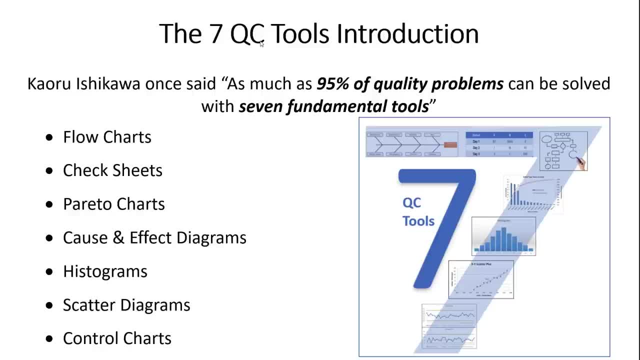 talking about green belt or black belt or quality engineering, it doesn't matter. These seven tools are incredibly powerful for solving problems and making improvements, And this is a really important topic. By the way, as we go through this, I'll make sure to talk about where we're. 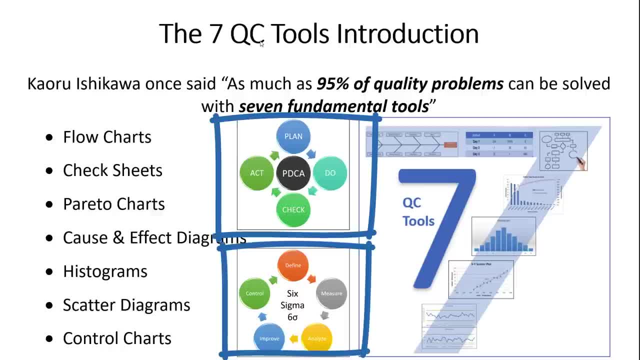 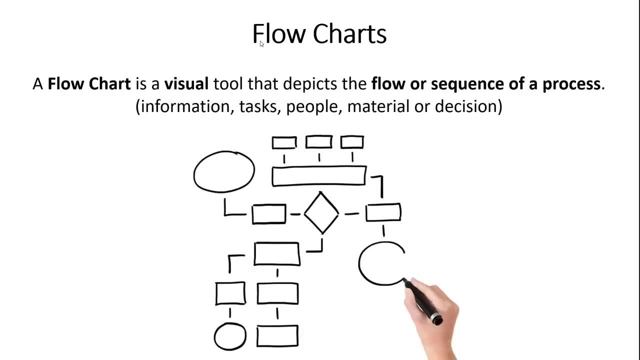 at in something like the plan: do check and solve. So let's get started. All right, let's get started. So let's get started All right, let's get started, All right, let's get started All right. so the very first tool is the flowchart, And what a flowchart does is 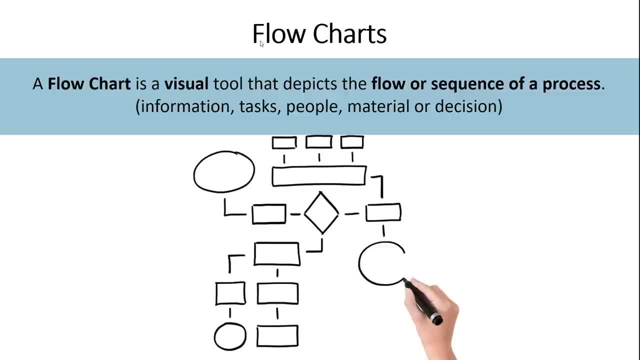 it's a visual tool that helps you depict the flow or the sequence of a process. This could be things like the flow of information, or the flow of tasks, or material, or people or decisions. It doesn't matter. The reason that a flowchart is so incredibly valuable is it makes a really complex. 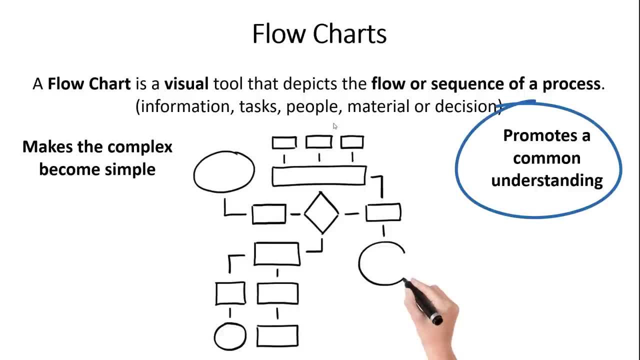 process simple and it promotes a common understanding of a process. Anytime you get more than one person in a room to talk about a process, there's likely going to be disagreement about how the process works, And I love using this analogy Oftentimes when we sit down to. 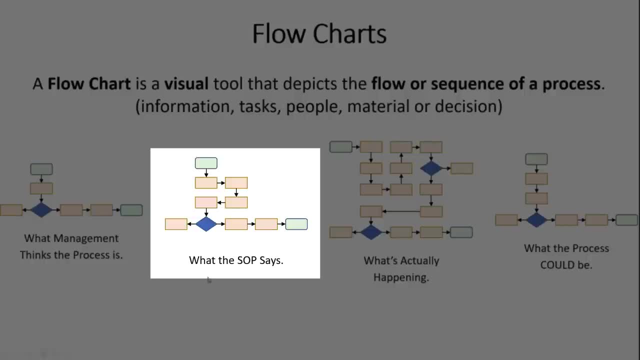 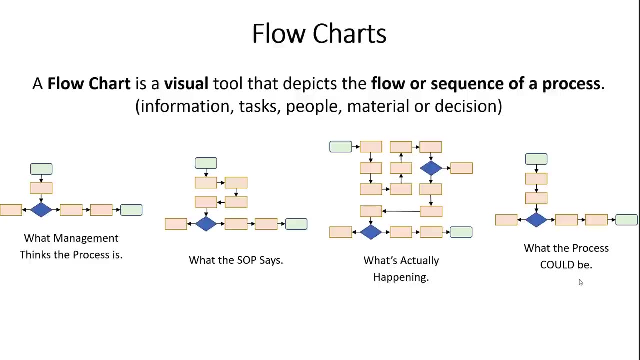 analyze a process. there's what management thinks is happening, There's what the procedure says is happening, There's what's actually happening on the production floor, And then there's what could be happening. And the beauty of a flowchart is it does just that: It gets everyone on the 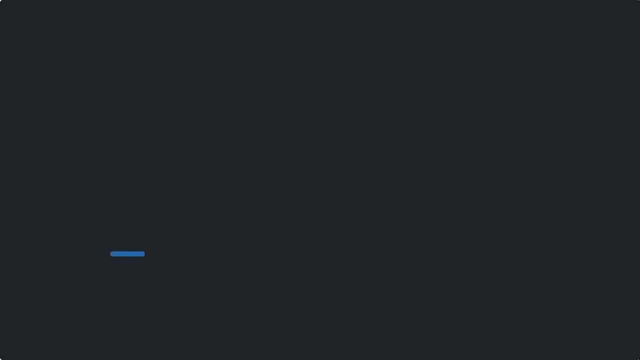 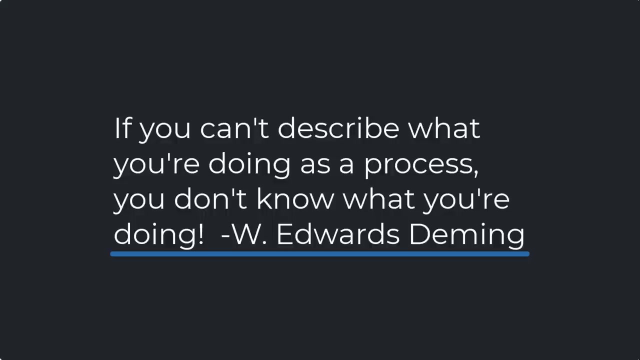 same page about what's actually happening, And I love this quote from Dr Deming, who said: if you can't describe what you're doing as a process, you don't know what you're doing. And the best way to describe what you're doing is to use a flowchart, And that's why this tool 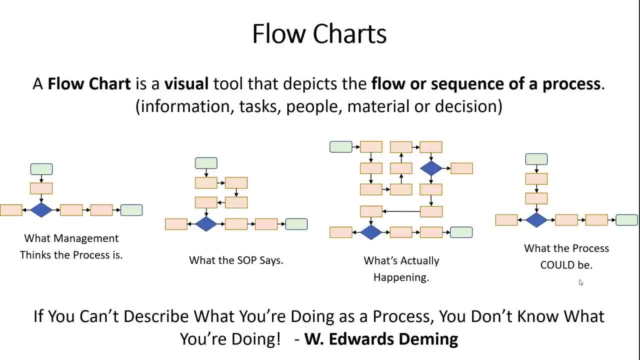 is so powerful. If you're in the planning phase or the define phase, it's really good to use a flowchart, define your process and then use that flowchart to plan out your experiment and plan out how you're going to make an improvement. So let's do just that. Let's say 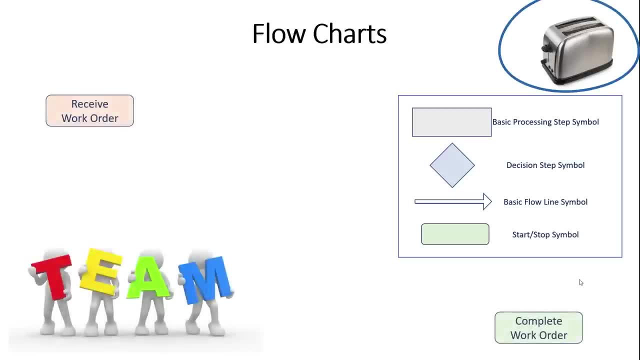 we're talking about our toaster and we want to make an improvement. right, And so the first thing we're going to do is we're going to start with the boundaries. We want to analyze a process, but we want to start with the boundaries first, So we're going to go from receiving a work order. 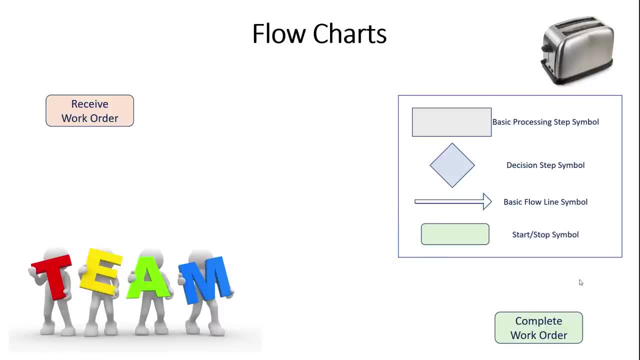 to completing a work order. That's the boundaries of our flowchart. Now I've got the team here, because all of these activities, all of these tools are all team-based. So imagine you're sitting down with your team and the first thing you're going to do is brainstorm all of the steps. 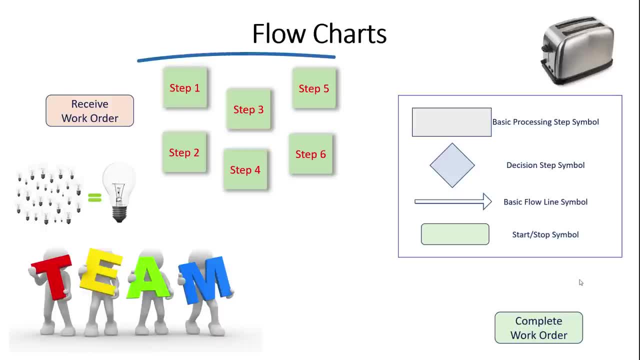 in the process, right. Talk to the experts. How does the process work? Use post-it notes, right? Don't try to do the same thing. Don't try to do the same thing. Don't try to do the same thing, Don't. 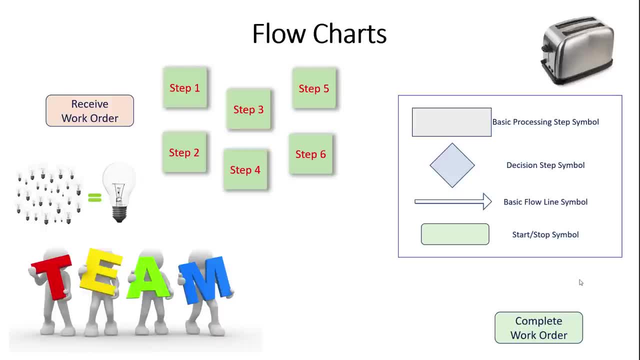 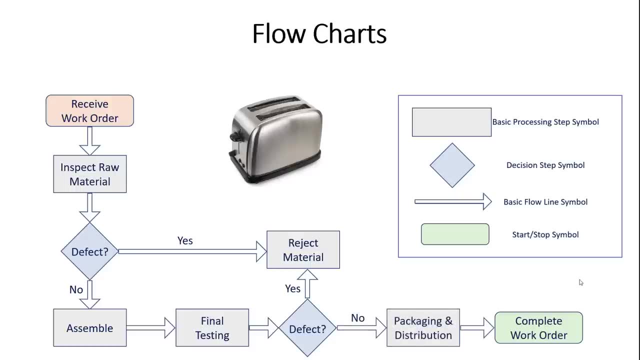 in some software use post-it notes, write down all the activities And then, once you're done brainstorming, organize those thoughts into that logical flow or that logical sequence of activities for your process. And now that we have our process here, we're in that planning phase. 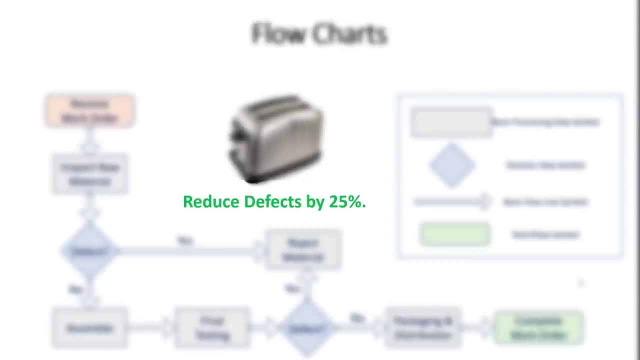 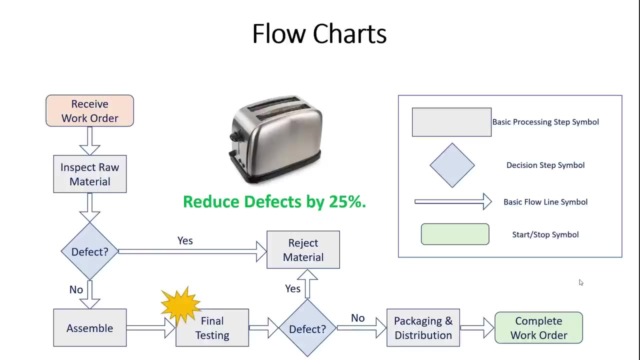 and we want to create a target right. What sort of improvement are we going to make? And we want to reduce defects by 25%. Now we can't make an improvement and we can't solve a problem without data And we know that most of our defects happen during final testing. 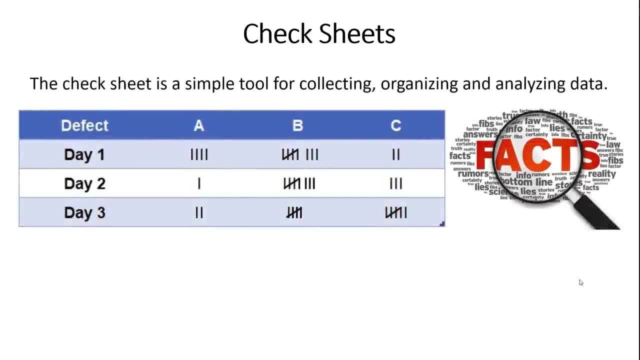 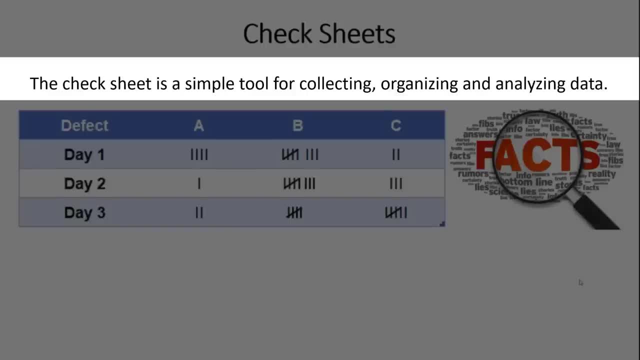 So now we need to make an improvement, And we need to make an improvement, And we need to make a little bit of data, And this is where the check sheet comes into play. So the check sheet is a very simple tool for collecting, organizing and analyzing data. Every problem you solve, or 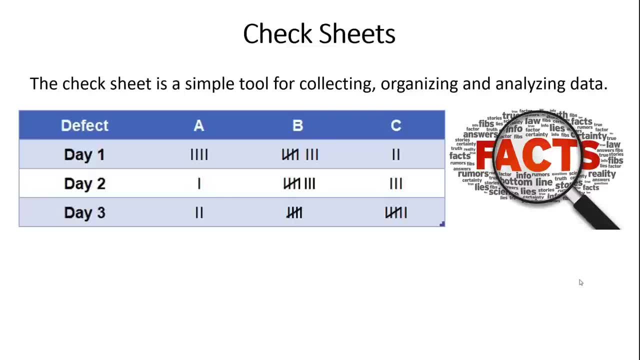 every improvement you make should be based on data, And the check sheet is probably the most powerful tool for collecting data. Now, there's something wrong with the check sheet that I'm showing you here on the screen, And that problem is is it doesn't have any metadata. If you're, 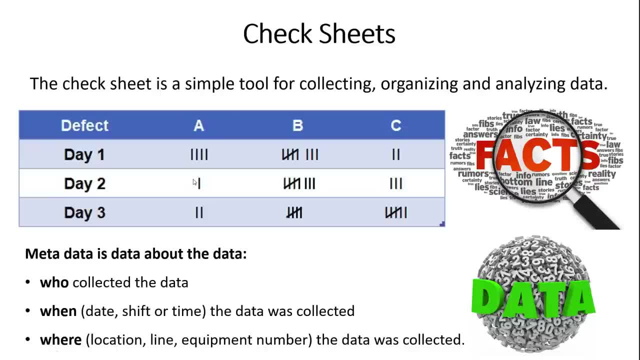 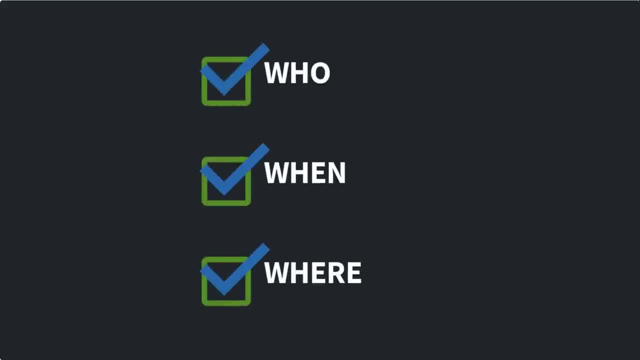 collecting data and you want to make a high quality decision using that data. you also need metadata, So when you're creating your check sheet, don't forget to include things like who and when and where. All those key elements of data integrity and data accuracy are really important for making 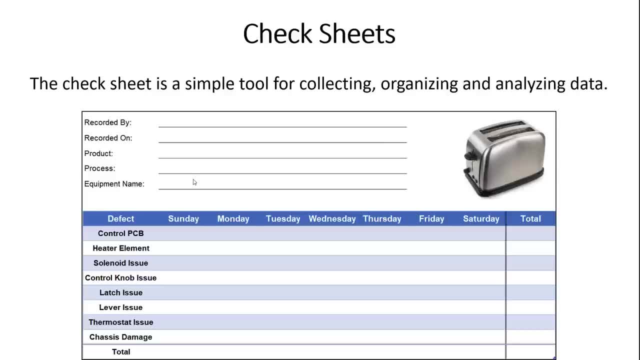 high quality decisions. Okay. so we've got the team together And again we did a little bit more brainstorming. We said, okay, at final testing, we have eight defects that we want to collect some data on, So we create this check sheet. we've got our metadata here, we hand this. 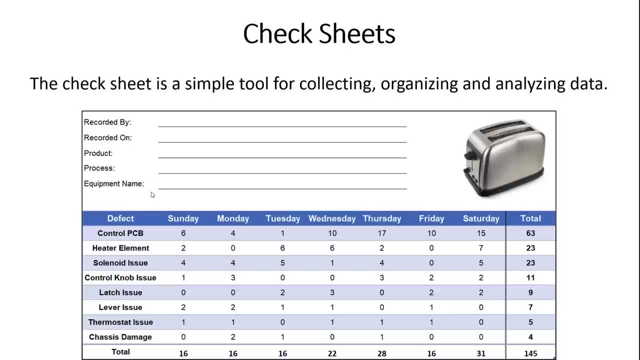 off to the team and they come back to us a week later with a bunch of data. Now this is fantastic. We finally have some data that we can analyze, And the question is: which defect do we focus on? I want to improve our target, So we originally said we want to reduce defects by 25%. Well, 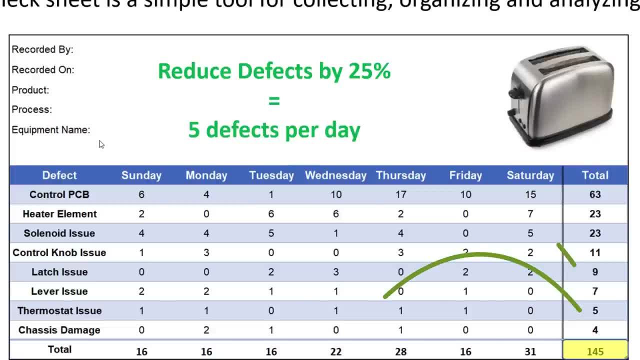 now that we have a little bit of data, we can actually create a target. So we have 145 defects across a whole week. that's seven days. That means we're averaging about 20 to 21 defects per day. Now if we can reduce that by 25%, we will eliminate five defects per day. 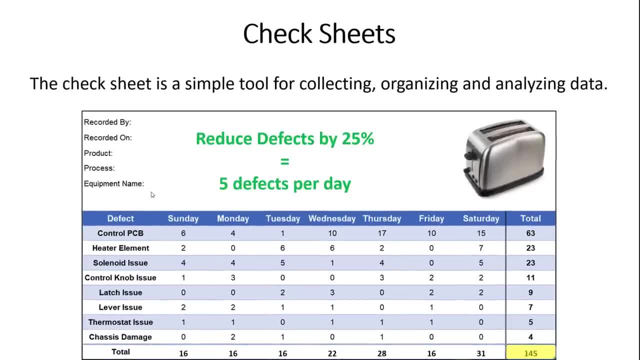 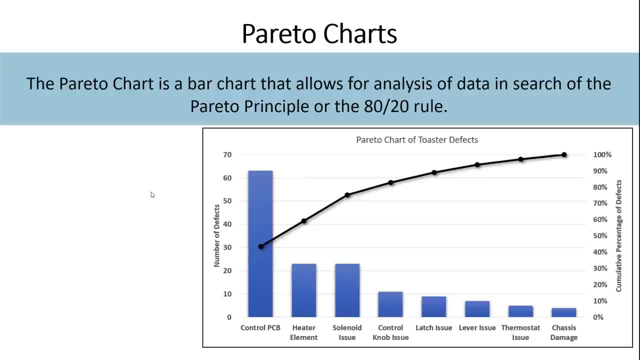 Now we obviously can't focus on all these defects, So the real question is: how do we know what to focus on? And that's where the Pareto chart comes into play. So the Pareto chart is another QC tool that allows you to analyze your data in search of the Pareto principle. 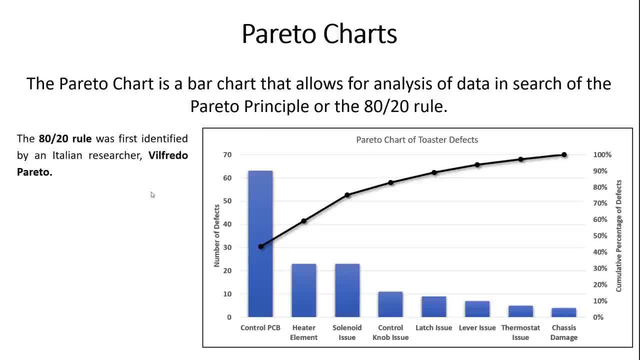 So what is the Pareto rule? What is this 80-20 rule? So this is a natural phenomenon that was discovered by a guy named Vilfredo Pareto. He's an Italian researcher who was studying land ownership and wealth distribution And he said: I want to improve my target, So I'm going to. 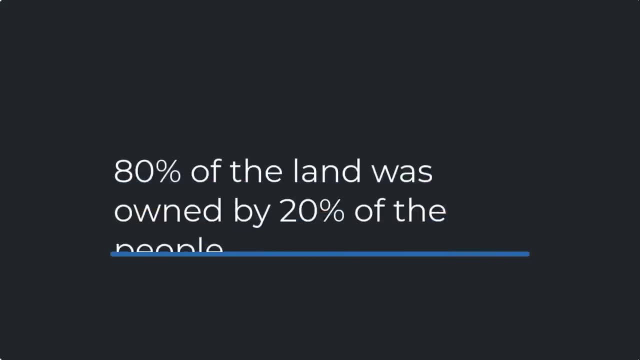 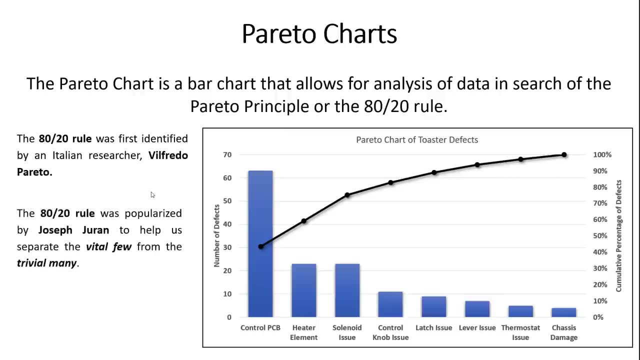 in Italy and in Europe, And what he found is that 80% of the land was owned by 20% of the people, And this 80-20 rule and this 80-20 phenomenon was also experienced by a guy named Joseph Duran. 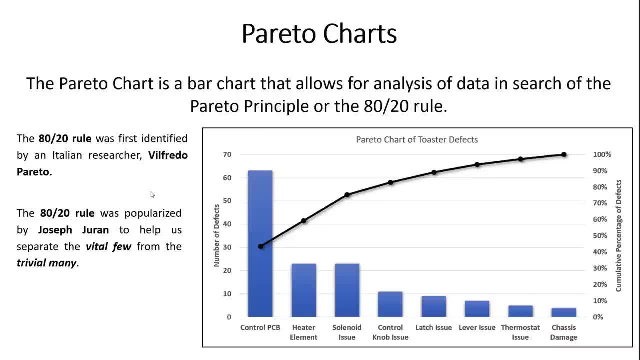 Now, he gave credit for the tool to Vilfredo Pareto, but he was the one who popularized this idea of the 80-20 rule and this idea of the Pareto chart And what he told us and what he taught us. 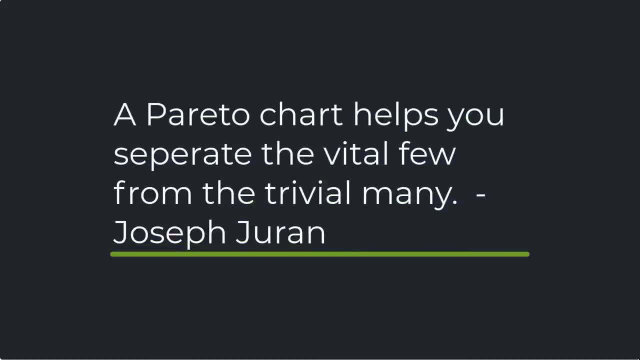 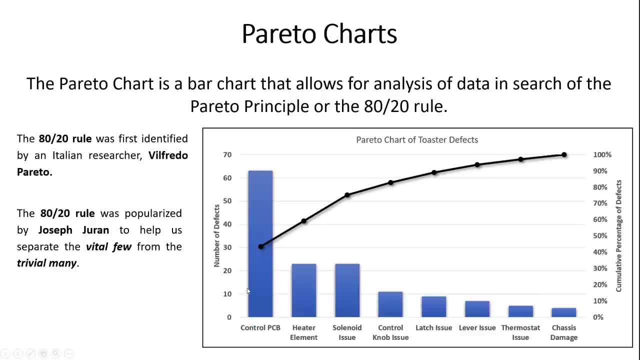 is that a Pareto chart helps you separate the vital few from the trivial many. Now, what did Duran mean? What he means is, when you're solving a problem, there's often one or two key issues, key root causes or key defects that you need to focus on to have a major impact on that particular. 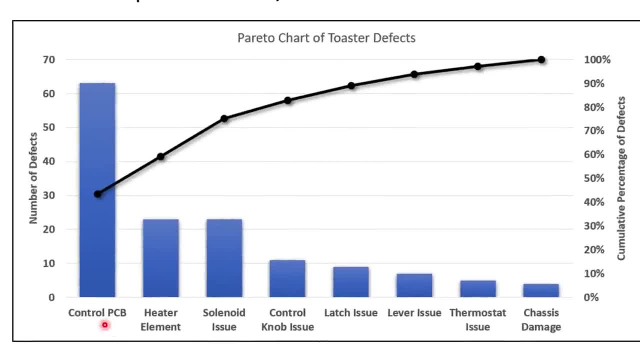 situation And that's exactly what you see here. When we take our data from the check sheet and we put it into this Pareto chart, we see that control PCB issues accounts for nearly 40% of our defects. You can see, if we come across here, we've got 40% of our defects coming directly from control PCB. 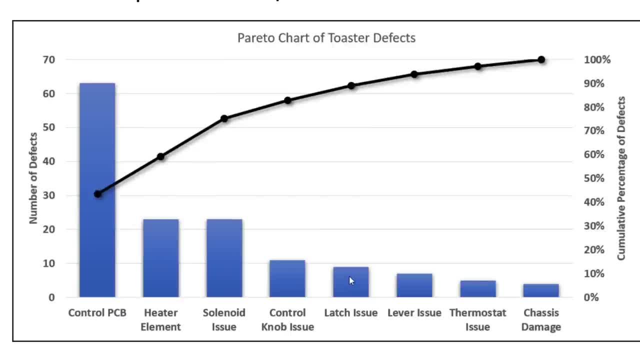 Now there's two things happening on this graph. Obviously, there's the blue bars, which are simply just the frequency or the count of defects that occurred throughout the week, And then this black bar is actually the cumulative line, So this first defect accounts for 40%, and 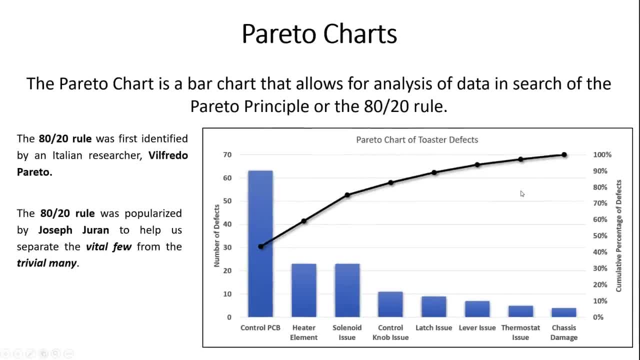 then we go up and up and up all the way to 100%. Now that we have this Pareto analysis, we know that control PCB is our primary issue. It tells us what to focus on. Now we still don't understand why these issues are happening, And this is where something like the cause and effect diagram can be. 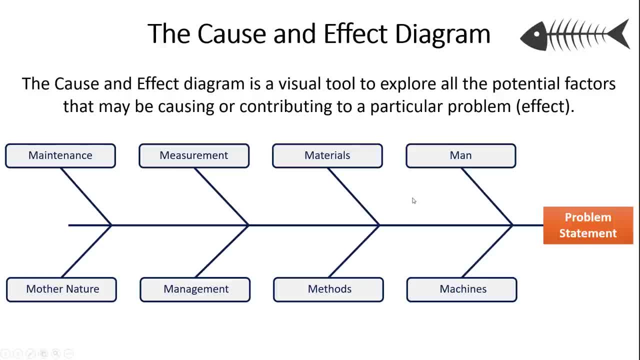 used The fishbone diagram or the Ishikawa diagram- there's all sorts of different names for it, but it is a cause and effect diagram, And the way this works is we start with the effect That's over here on the right, That's the head of the fish here in orange. This is our effect, And so step 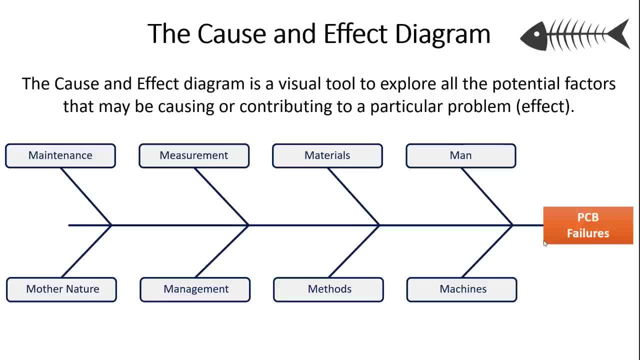 one of the cause and effect diagram is to start with a really well-written problem statement. So I put in PCB failures, but in reality you want to have a much more descriptive problem statement than this And once you have this effect you can start working through the fishbone process. 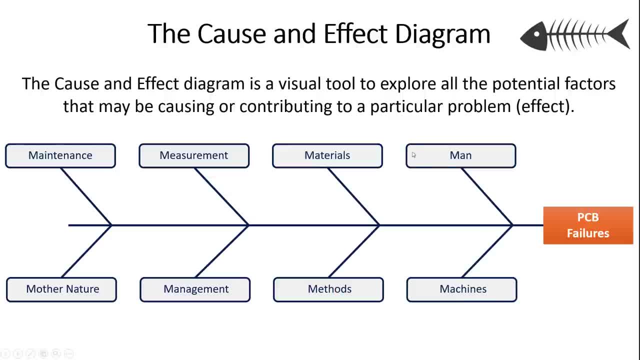 to analyze all of the potential causes and failures. Now I'm showing here what's called the 8Ms, And this is the beauty of the fishbone process is that it's a well-structured approach to root cause analysis. It forces you to think about all of the potential different categories. 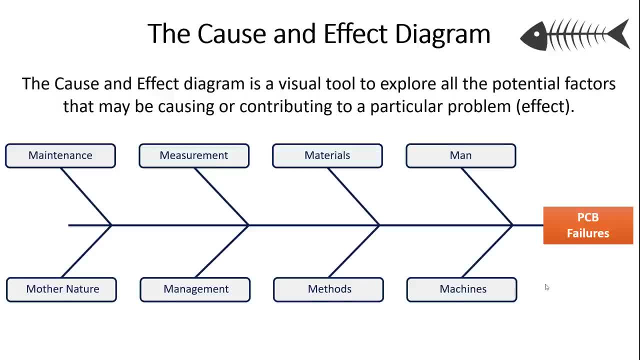 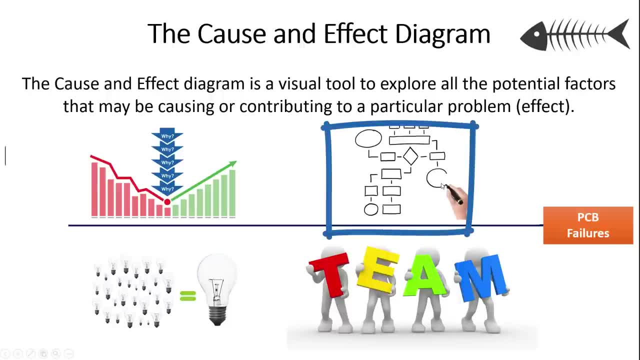 or scenarios or causes that might be contributing to your problem. Now, along with the cause and effect diagram, are a number of tools that you should be using, So I would recommend you get out your flowchart, look at your process, use your flowchart and then start working through the 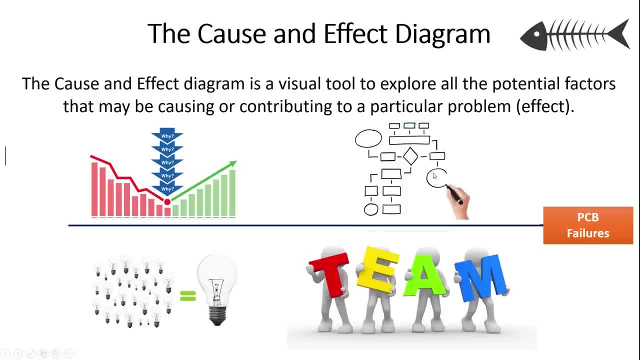 and ask yourself how might each step in the process fail and contribute to the effect that we're seeing? Teamwork is also a must here. You're not going to be a subject matter expert in all of those 8Ms and you need people from operations and engineering and quality and R&D and marketing and 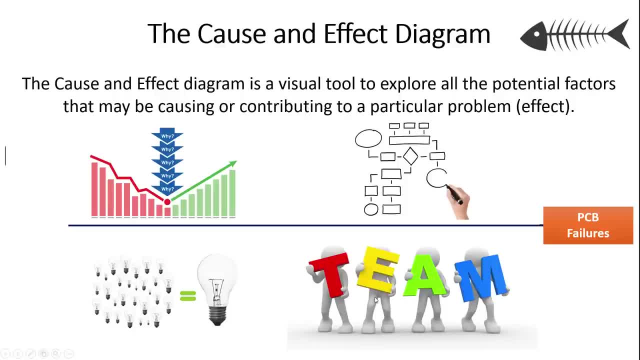 maintenance, to really do a thorough analysis in each of those areas to truly understand the root cause. And then, of course, brainstorming: You're going to have to creatively think about and talk about and discuss potential root causes. And then the 5Y analysis. I love the 5Ys. It really helps you go from a high-level symptom. 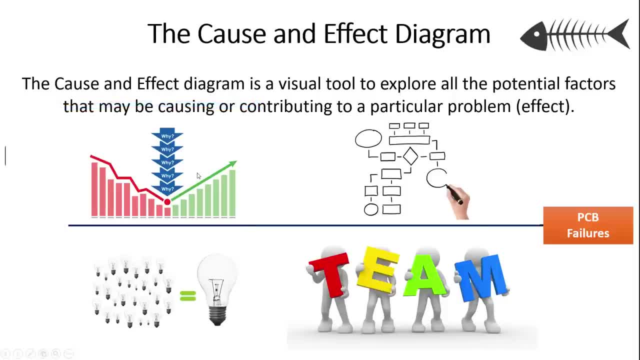 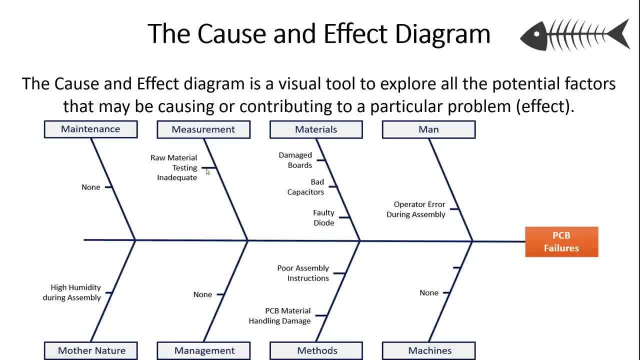 down to the true root cause and really ask: why, why, why? to truly get to those real root causes that you need to address. And then, as you have that team discussion and you go through the process, you can identify potential root causes and contributing factors to the problem you're. 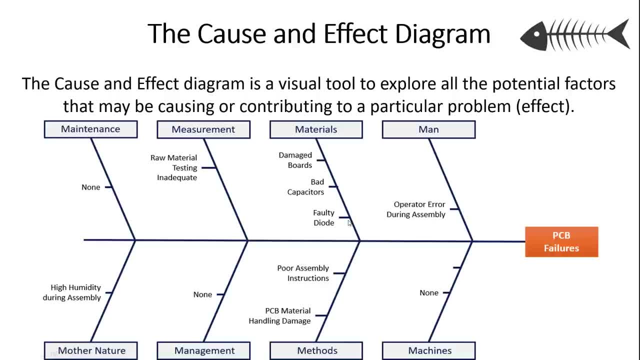 trying to solve. Now, obviously, again we have to go back to that pretty principle. We can't focus on everything. We have to talk about the most likely root cause And then, as you go through causes and the most likely contributing factors. So again at the end of your cause and effect. 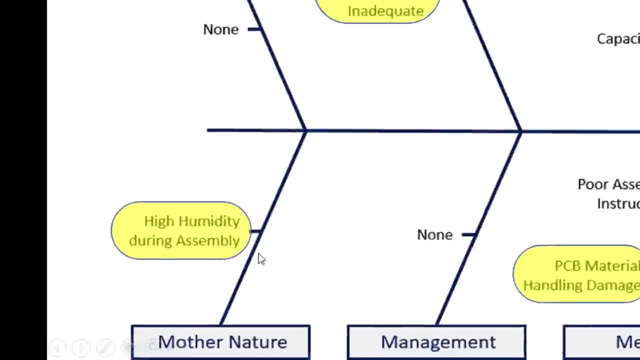 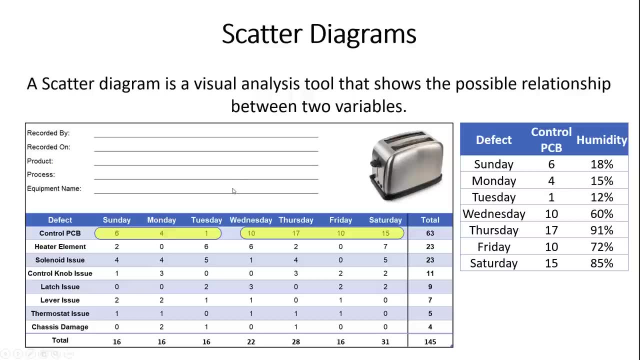 diagram, you might identify three or four issues that you need to study further. Now I want to talk about this one: high humidity during assembly. Now, as we were working through the cause and effect diagram process, the engineer who was helping us looked at our check sheet and noticed: 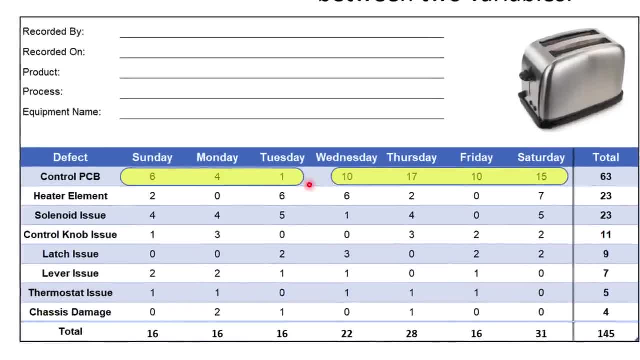 an interesting pattern. What they noticed here, and I've highlighted here in yellow, is that Sunday, Monday, Tuesday, we only had a few defects- right, Six and four and one, Whereas on Wednesday, Thursday, Friday, you'll notice that we only had a few defects. So we're going to talk about 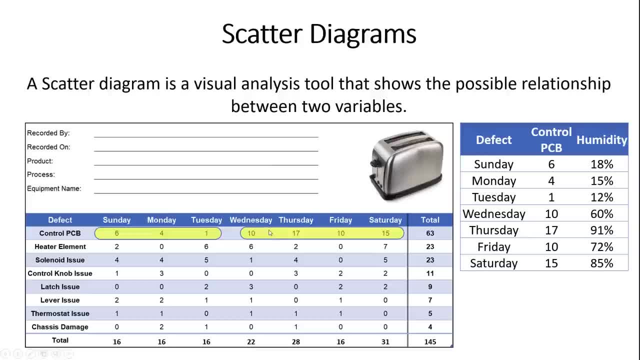 notice that our defect rate jumped up a little bit, And what the engineer remembered is that we had a rainstorm come through on Tuesday night and the humidity level in the facility really jumped up. And so what? the hypothesis here is that humidity is affecting our defect rate. So 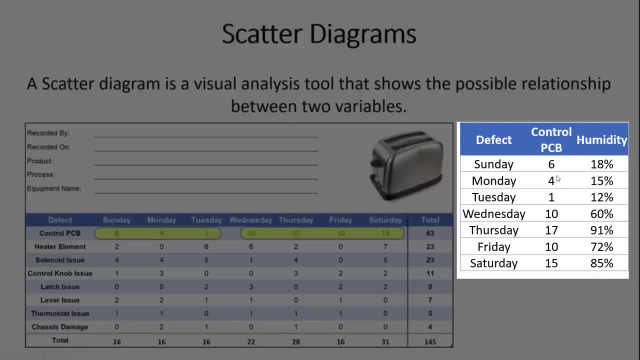 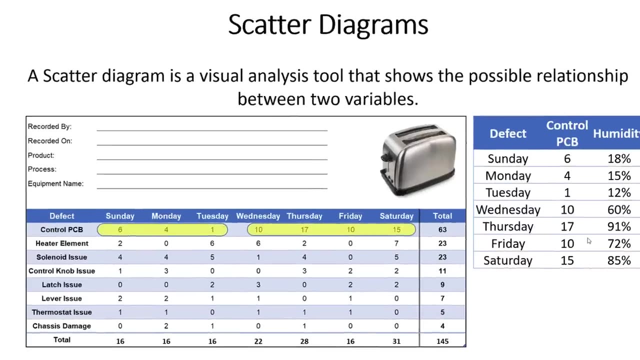 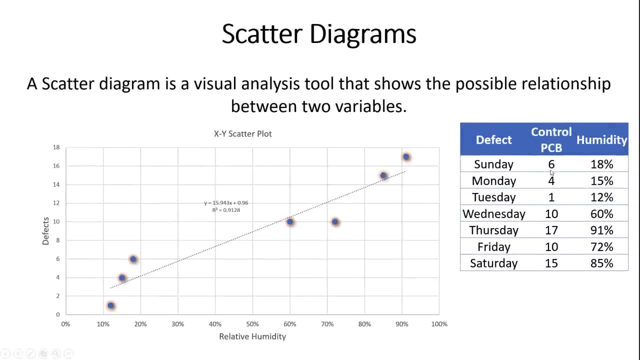 I've created this little table here to show the days of the week, along with the defects and the humidity. Now, to truly understand this relationship, we have to create a scatter diagram. So here's exactly what that scatter diagram looks like. What we do here is we're plotting pairs of data. So, for example, on Sunday we had six defects. 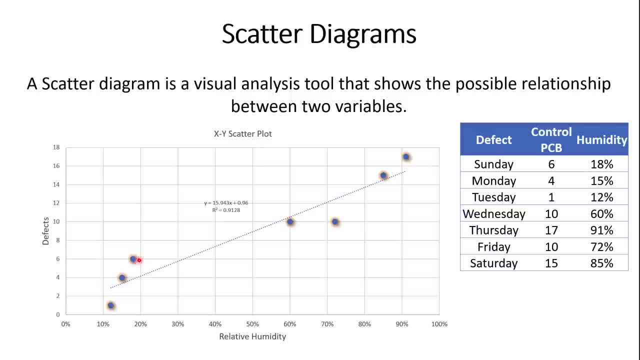 and 18% humidity. You can see that right here. That's this data point. right here We had six defects: 18% humidity. Now, the way this scatter diagram works- or you might hear this called an X-Y scatter plot- is here: on the X-axis, we put our controllable variable, our independent variable. 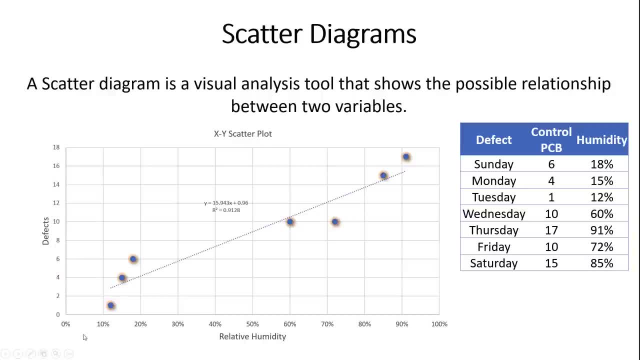 and then on the Y-axis we put our response variable. So here we believe that relative humidity is the independent variable that is affecting the data. So we're plotting pairs of our response variable, which is defects, And you can see here that there appears to be some. 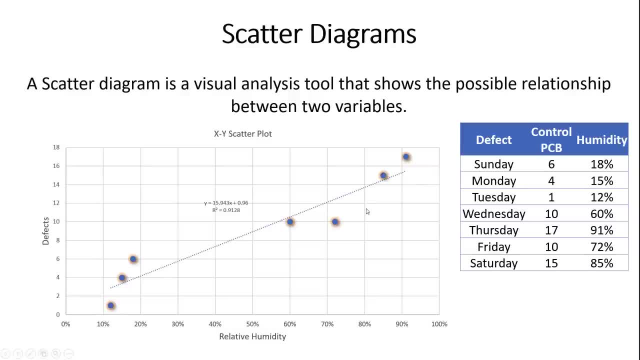 relationship between PCB failures and humidity. Now, it's really important when you're looking at the scatter diagram, not to assume that this relationship is a causal relationship. right, There's this really important concept that you can have correlation without causation. Two parameters or two variables can correlate without having a cause and effect relationship. 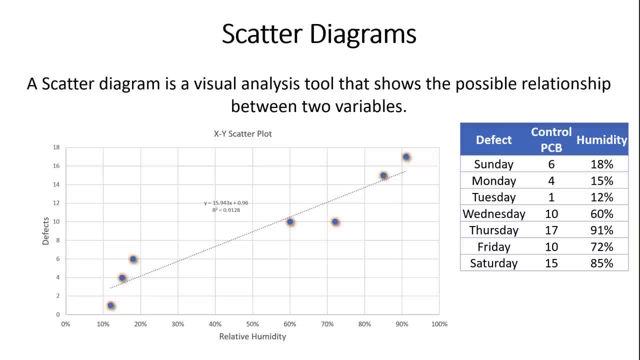 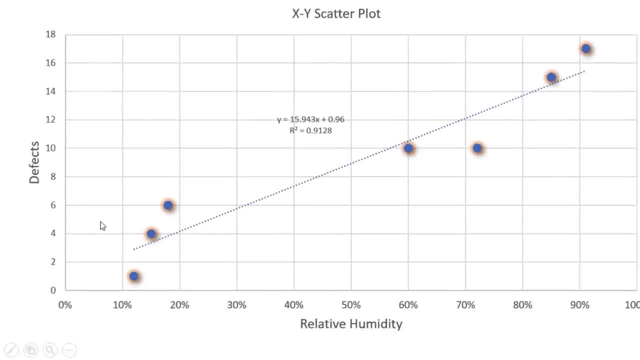 So let's assume, though let's assume- that we've done a DOE here and we've proven that humidity has an effect on our PCB defects. We could come back to the scatter diagram. We could say: okay, our target for PCB defects is five or less. Let's call it five or less. 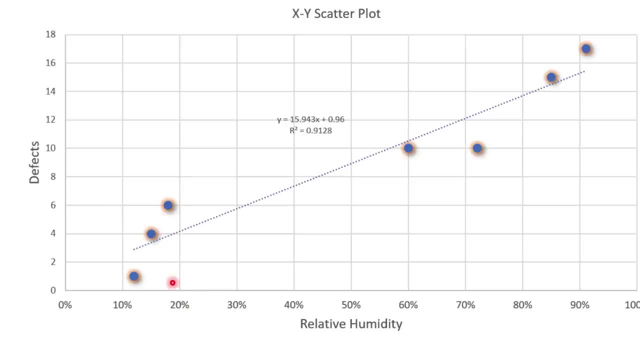 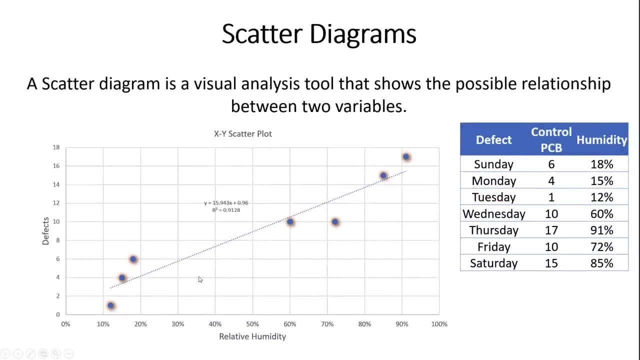 And so we come down here to humidity and say, okay, we want to control humidity to around 20% to keep our defects low. Does that make sense? And this is a great way. a scatter diagram is a great way to understand the relationship between two possible variables. Now, once you've done your, 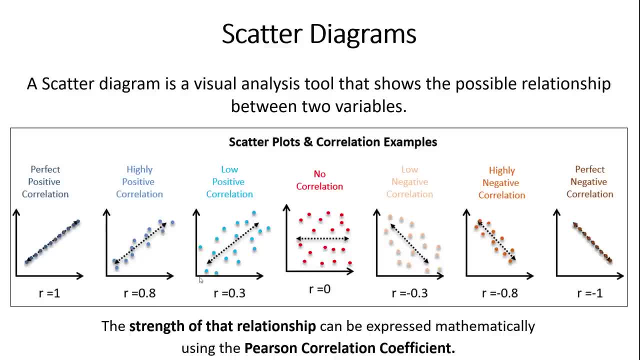 scatter diagram, you're going to be able to see that there's a relationship between two possible variables. You can quantify the relationship between those two variables. So what I'm showing here is the Pearson correlation coefficient, And this coefficient ranges from positive one all the way. 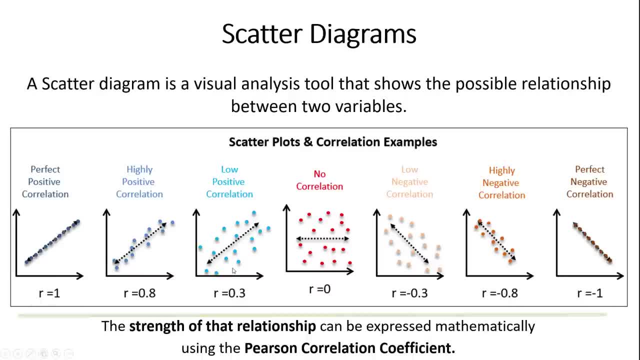 over here on the left to negative one all the way over here on the right, And that ranges from a perfectly positive correlation. here You can see that as X changes, Y changes identically, And then same thing here with R equals minus one. This is a perfect negative correlation. Now, as we get, 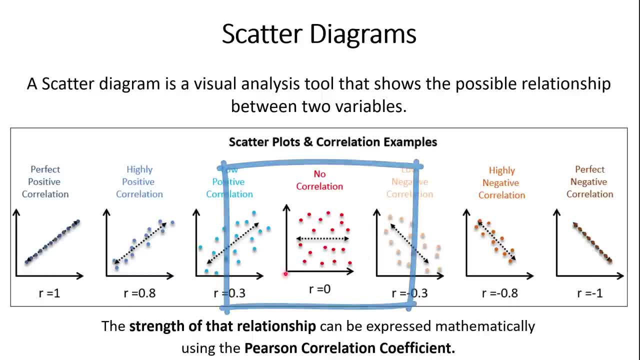 closer to zero, we start to lose that relationship. So an R value of zero means that we're going to have a relationship between those two variables. So what I'm showing here is that there's no correlation between those two parameters. As X changes, Y basically does whatever it wants. There's no 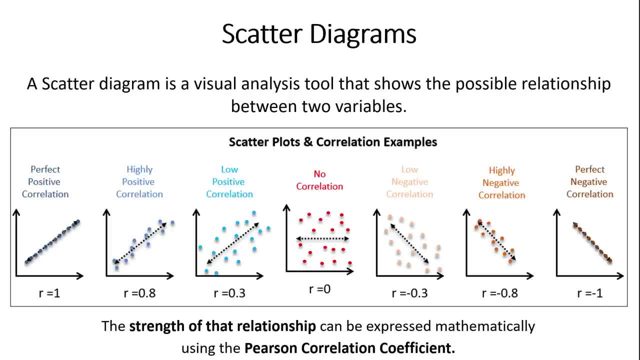 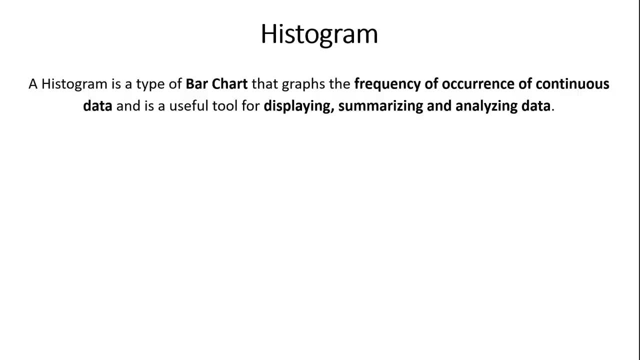 relationship between those two variables. Now the next thing we could do in our analysis is to look at relative humidity over time. So let's say we go out, we talk to our facilities engineers, we say, okay, give us the relative humidity within our environment, you know. 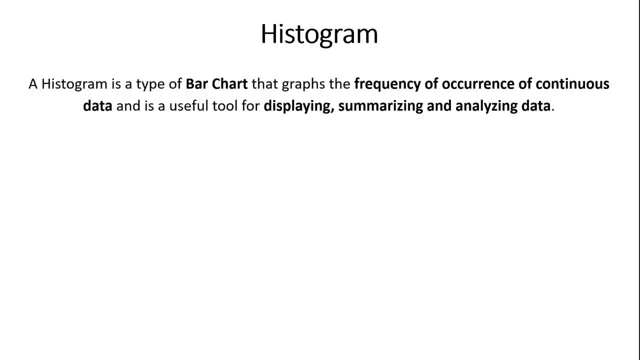 every six hours for the last six months And we can take that data and we want to plot it because we need to understand how relative humidity is changing within our facilities. So we're going to, and one of the ways you could analyze that data is with a histogram. So a histogram is just a very 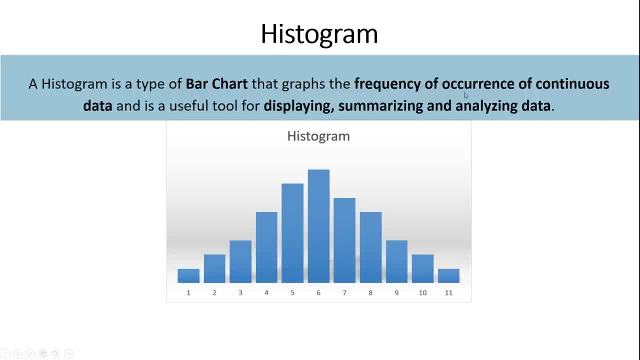 simple bar chart that graphs the frequency of occurrence of continuous data. And again, this is a great way to talk about your process. Every process or every product or every quality attribute out there has some level of random, normal variation. that will often occur in a pattern And as 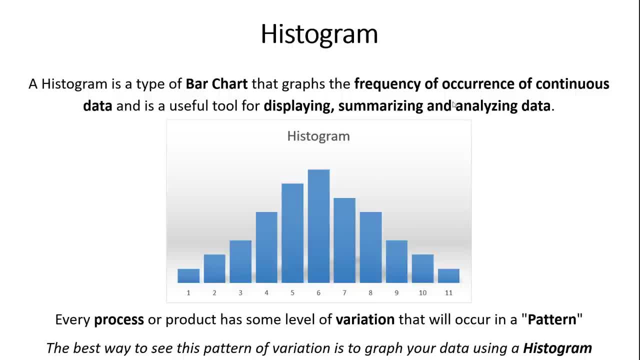 engineers, we need to understand what is the pattern associated with our outputs or our process, And a histogram is a great way to understand the pattern or the variation in your process. Now you might grab this data and you might get like a skewed distribution or maybe a bimodal. 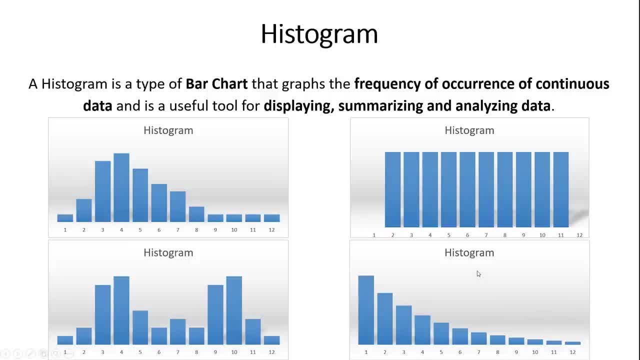 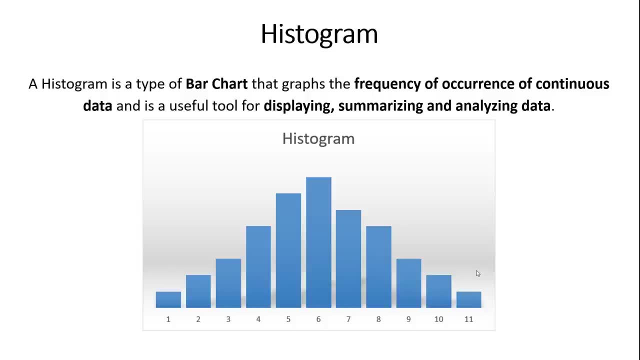 distribution or exponential distribution. There's all sorts of distributions you might get, but it's great to know how your process is behaving Now. the other beautiful part about a histogram is you can take this data and let's overlay some specification limits right Now. 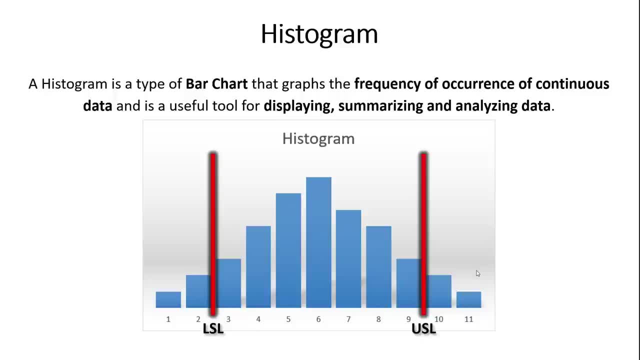 what we have is the beginnings of processes. So let's say we have a histogram and we have a capability. So the histogram is a fantastic tool to quantify and understand how your process behaves. And if you compare that against the specification limits, we can now start talking. 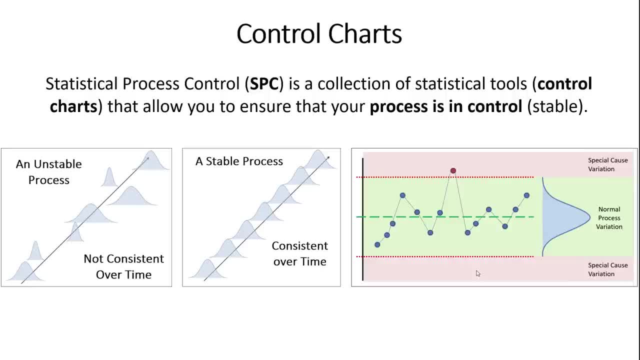 about process capability. Okay, So we're on to the very last and final QC tool. Let's assume we now control for humidity and we want to make sure that that change has been effective over time. A control chart is the right tool, or the perfect tool, to do that. So what is a control? 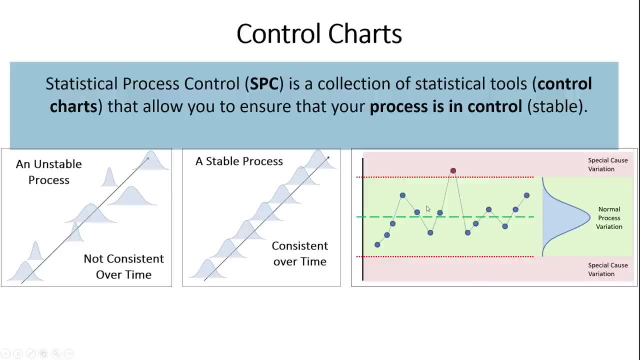 chart. It is essentially a tool that allows you to control your process. So let's say, you have a process that is in control. Now, when I say in control, what I mean is that you're only experiencing normal variation When your process is experiencing normal. cause: variation: your data. 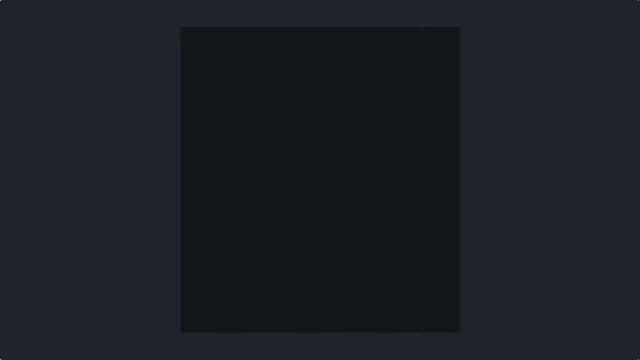 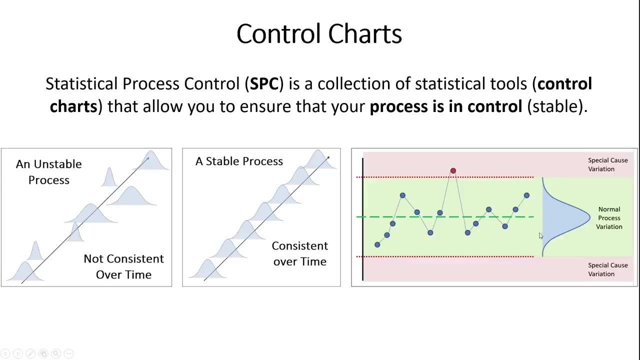 should fall within those control limits. By the way, if you're new to SPC, I have a whole separate video on control charts. You can go check it out. I've got both the X bar and R chart, as well as attribute data, And a control chart is a fantastic tool to use at the end of a project to monitor and 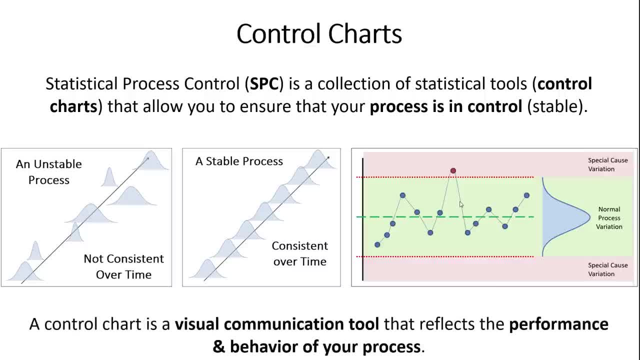 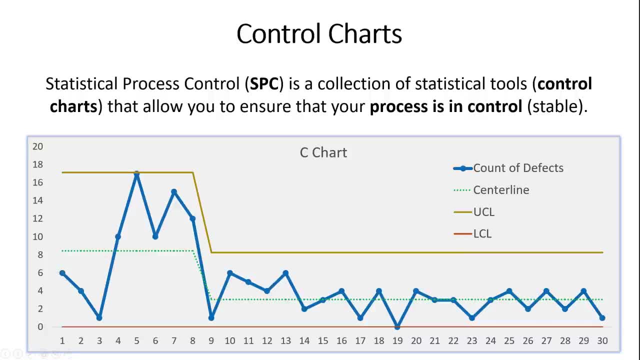 control your process and make sure that your changes were effective. And let's take a look at what this looks like for our particular process. So here's our process right- The first week of data. you can see we're really all over the place and our control limits. 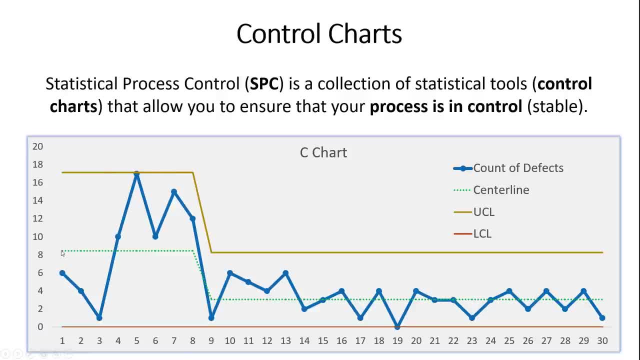 are really wide because we're not controlling for humidity And we've got all this data and you can see, on average we have about eight defects per day, right, And we're really jumping around here. And then, let's say, on day nine we start controlling for relative humidity and we've 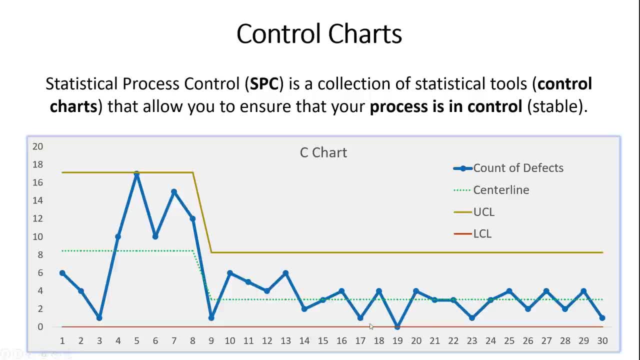 got our control chart and we're collecting data And you can see that for the next 20 plus days our defect rate has increased. So we're really all over the place And we've got all this data dramatically fallen. In fact, our new mean defects per day is around three. So essentially,